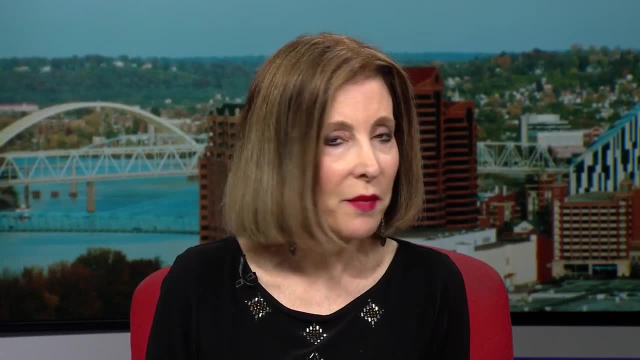 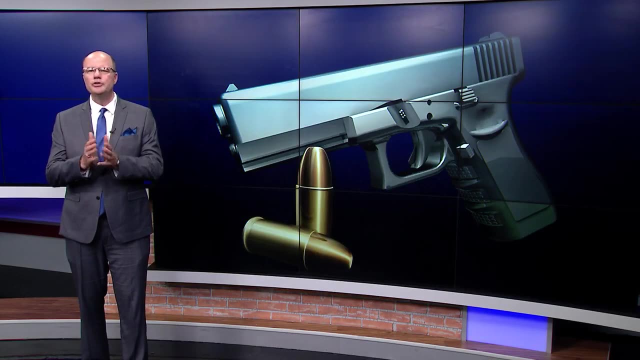 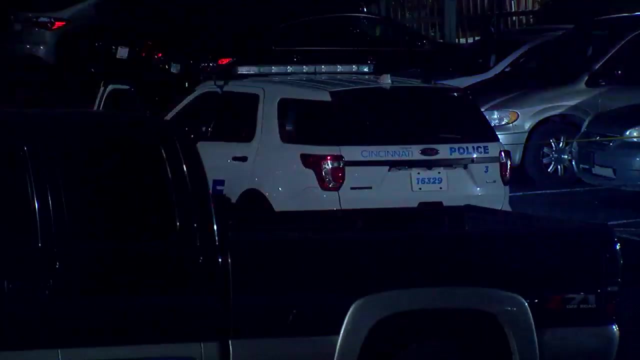 COVID pandemic hit Now. new research from the CDC demands our attention. Local 12's James Pilcher is here with numbers that have people talking, James. Yeah, thanks, Paula. The huge increase in lives lost is felt in Cincinnati and around the entire nation, And it's not just limited to big cities. The Centers for Disease Control and Prevention found gun deaths from either homicides or suicides surged in 2020, the first year of the COVID-19 pandemic. The study is part of a 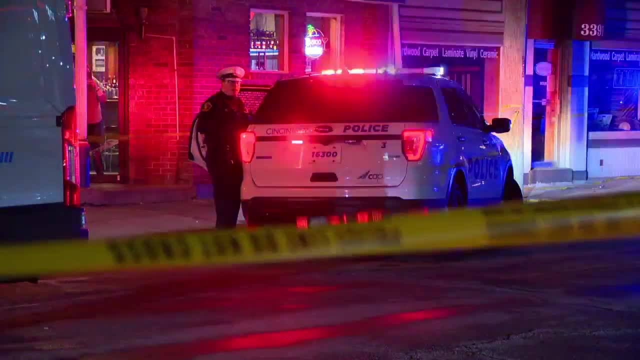 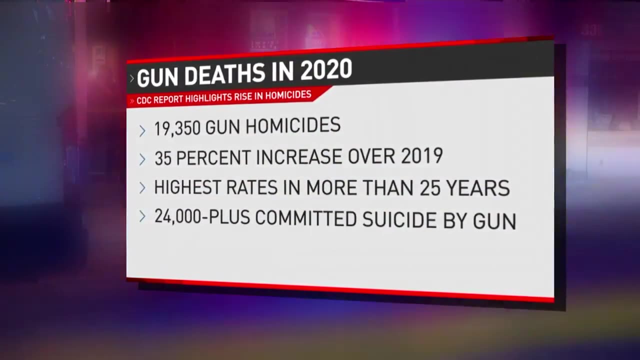 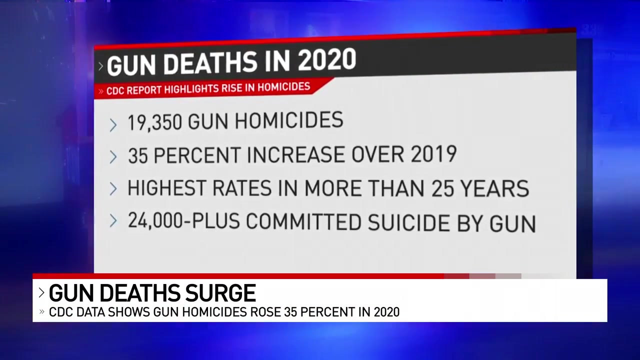 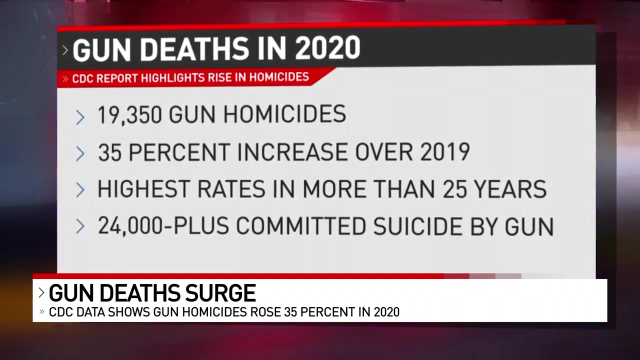 newly funded effort to study gun violence and its impact. The researchers found homicide rates by gunfire climbed to more than 19,000 in 2020, with urban and rural areas both seeing startling increases. The total is up 35%, or nearly 5,000 deaths, compared to 2019.. That number is the highest in more than 25 years. 24,000 people took their own lives using a gun in 2020.. The CDC's Dr Deborah Ori. 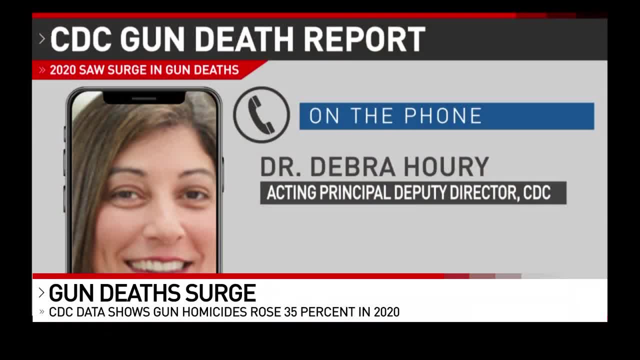 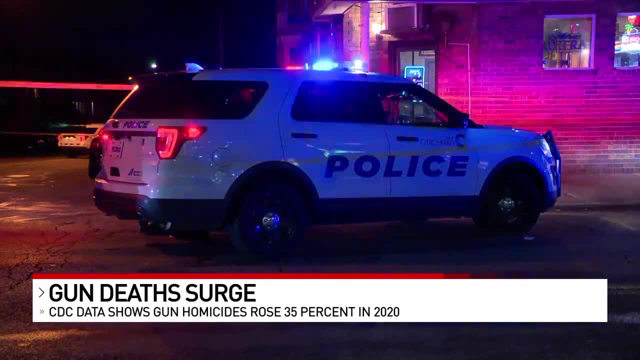 knows the damage bullets can do. Firearm injury is, tragically, a major public health problem in the United States. As an emergency room physician, I saw firsthand the pain and destruction to families that firearms can cause and why we must prevent these injuries. 3,735 black males between the. 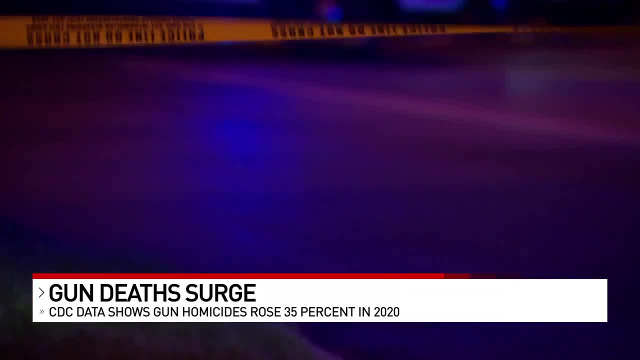 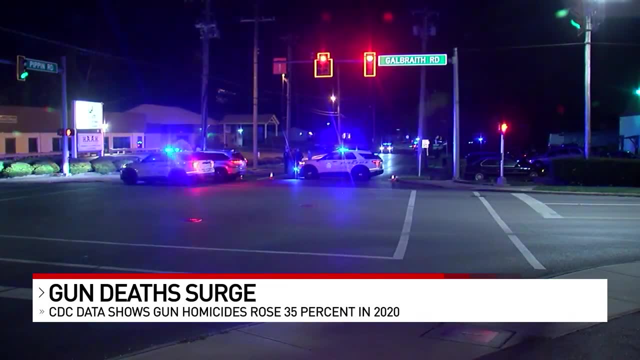 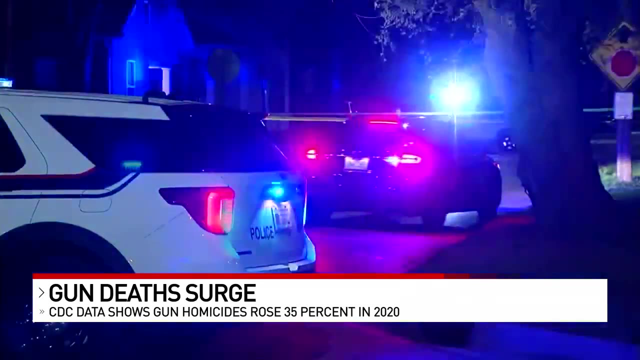 ages of 10 and 24 died after someone else shot them in 2020.. The group saw the largest rating increase. A black male between 10 and 24 was 21 times more likely to die this way than a white male in the same age group. The report suggests better funding for several possible antidotes. 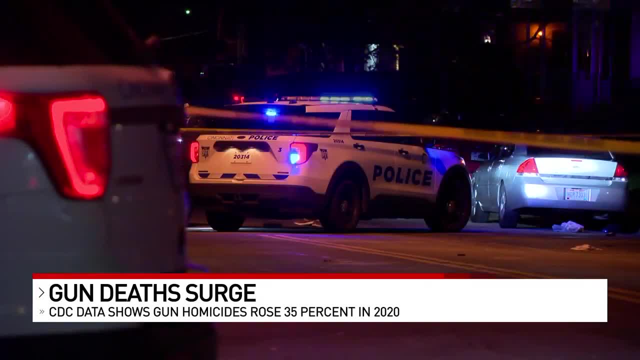 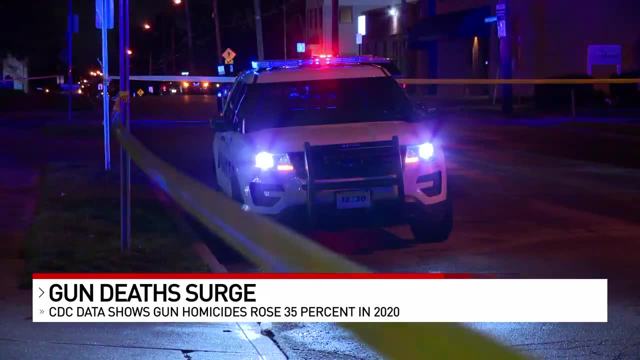 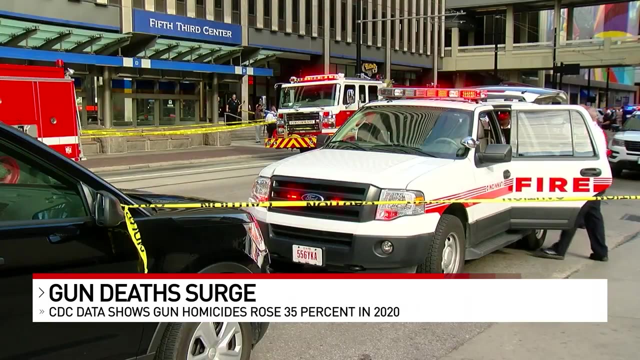 including more anti-violence workers on the street, more counseling services and even green spaces to better improve access to parks, But it stopped short of addressing gun control. Whitney Austin survived a mass shooting at Fifth Third Tower in 2018.. She since began. 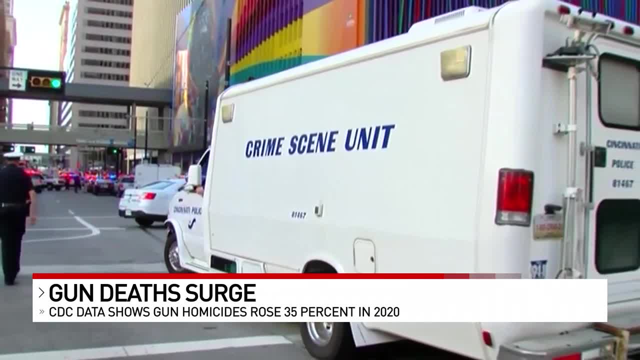 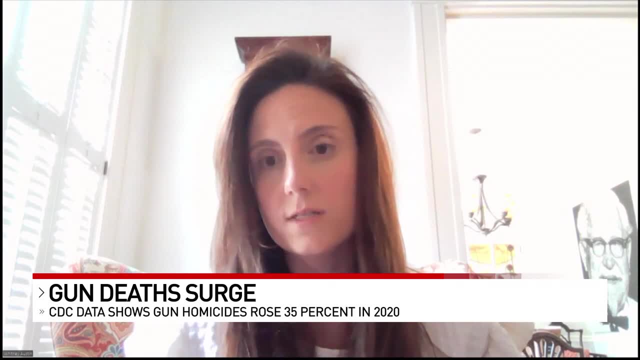 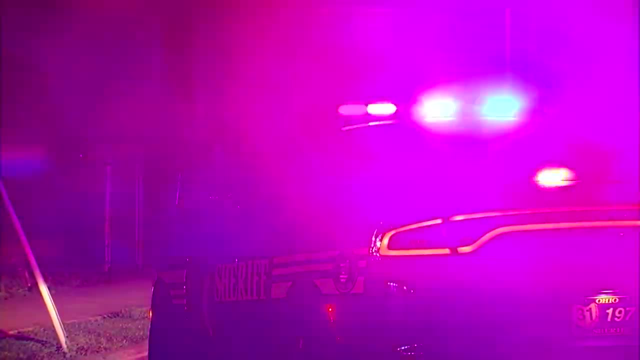 a non-profit aimed at reducing gun violence. It was the most violent year on record in the history of CDC numbers And to start, that's really hard to hear as a victim of gun violence. Legislation is important to focus on, but we also have a many number of solutions.